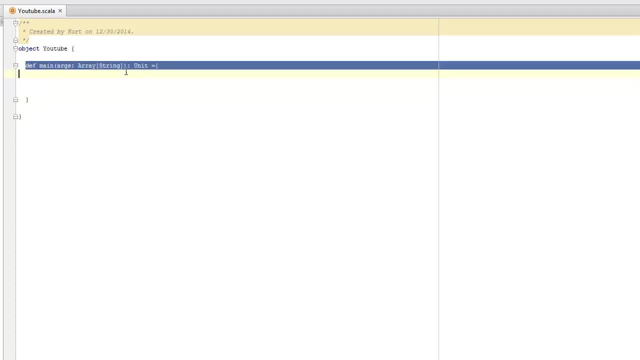 It's just kind of a standalone thing. For example, this main thing right here is a function, but it's part of the YouTube object. A function is just kind of on its own and I'm going to show you how to write those, which turns out to be the same way as how you write a method, but we'll get more into all that kind of stuff later. 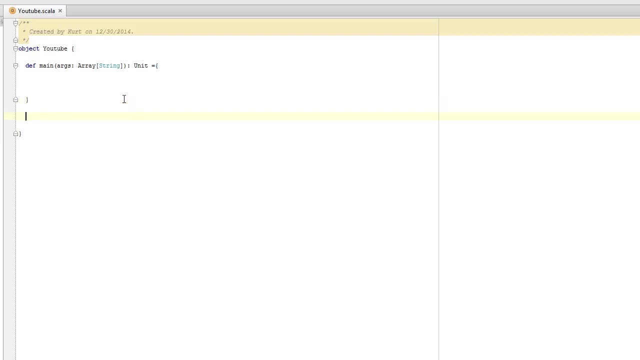 So what we're going to do is, after that last curly brace from the main method, I want you guys to make a couple of new lines to give us a fresh start, and we're going to type in a function that allows us to add two variables together. 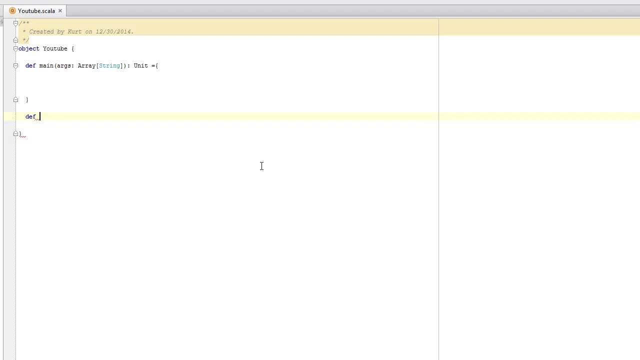 So to do this, we just We're going to say def, which stands for define, add, which gives us the name, and then parentheses. Now, in the parentheses, we want to say the variables that we're using. Kind of name them for the rest of the method. So we're going to say a- int because we're going to make an integer called a, and then we're going to say b- colon- int because we want an integer that we're going to call b. 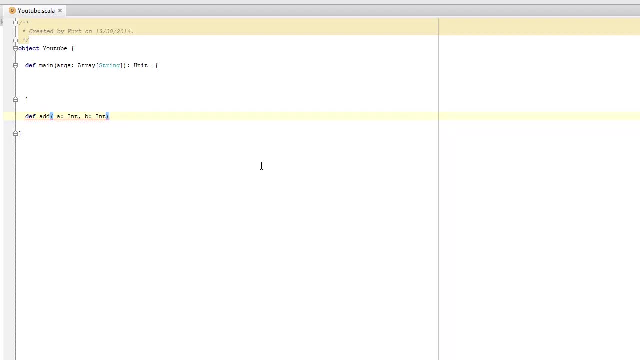 Now, outside of the parentheses, is where we define the return integer to get the return number from the box. We're going to fill that in Just to make sure you see the right distance type or the type of the function. so it's the same kind of syntax as we did for. 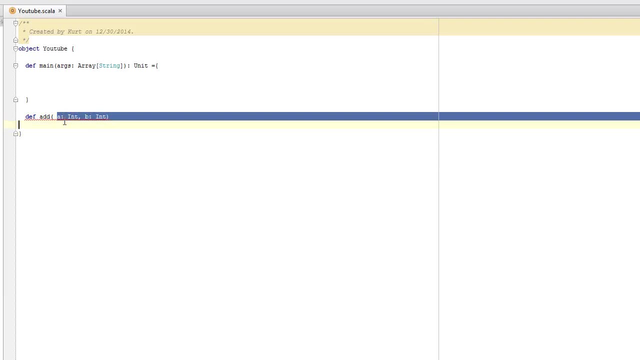 the variable or, I guess in this case the value. a colon int says that it's of type integer and it's the same thing for method. you say int, then you just say equals and curly braces, and you'll see, there's a really close relation between how we wrote the main function and how we're writing the add function. so now, 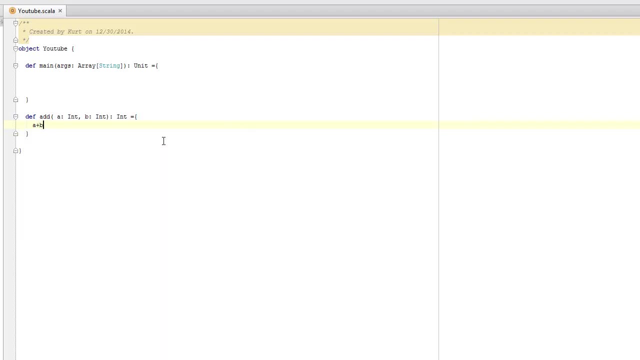 let's actually add these two together. if we say a plus B, we've now added the two together and the value is returned to anything that is calling this function add. so now that we've defined it, it does everything that needs to do. we can actually call it up here in the main method. 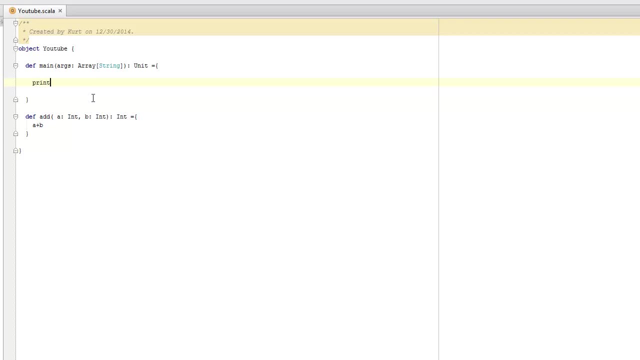 and see what value it sends out. so we're going to just say print line and then add four and three. now, if we save and run this, we'll see that we get the output of seven. if you're coming from java, by the way, too, you may notice that this is strange because we don't have a return, and i'll talk about. 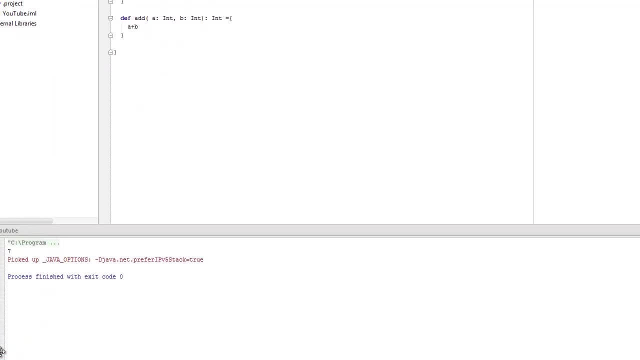 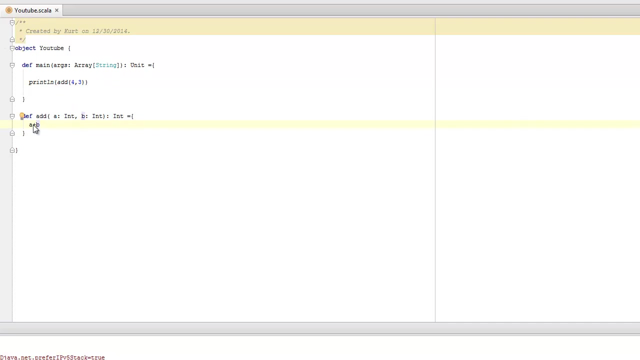 that in just a second. so if we go up here we see seven was printed out. so we have our value of our method, perfect. that's what we expected. we didn't get some other kind of strange number, so everything's working as planned. now, like i said, if you came from java, you you might be wondering. 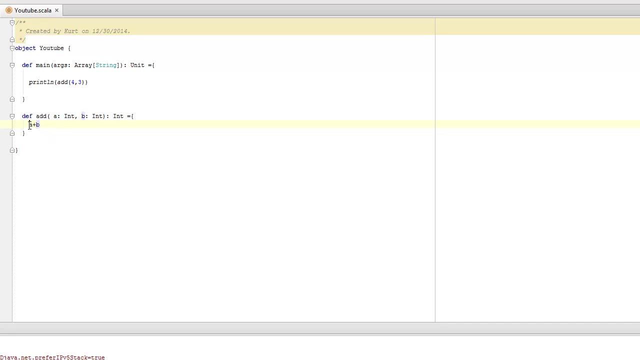 well, that's really strange. usually you have to say return type or return the value, otherwise you also get an error saying that this doesn't return the same type as what the method says it's going to return. well, in scala you actually don't have to worry about that. you can if you want to. it's an optional. 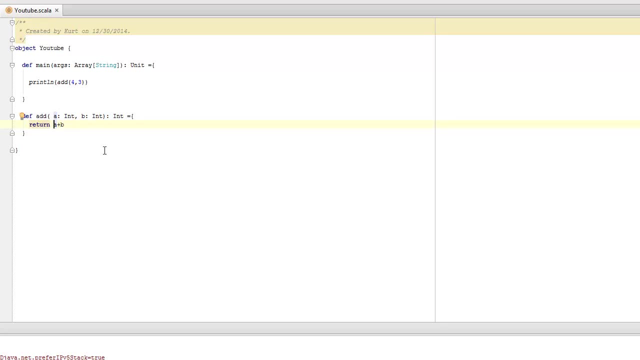 thing. you can say: return a plus b, and that will work just as well. but in scala the method will also return the value of the last expression. so in this case the expression a plus b is seven. when we give it, a equals four and b equals three. 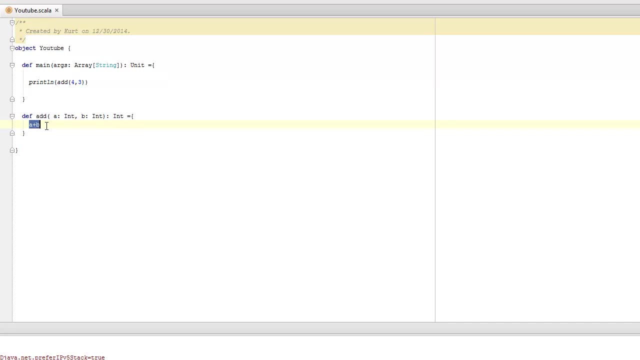 so there's no need to say return a plus b, because the last expression in here is already an int value. a plus b is going to return that value, and so there's no point in having to explicitly say return a plus b for no reason. now we can also make another method. let's call this one. 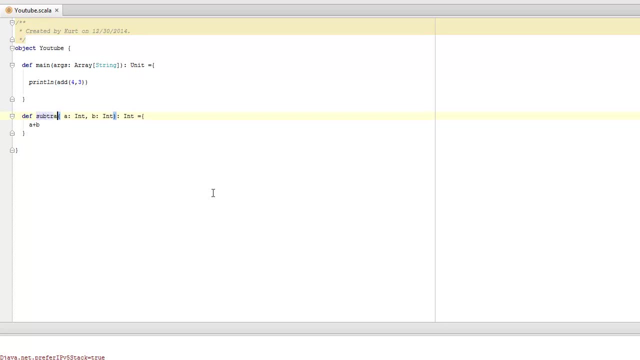 uh, subtract. we're going to be unique here and we can say, uh, a colon int, b colon int, and then let's say c colon int, so the integer c, and we can actually just subtract c from this value, and you'll see that we still, as long as we change our method up here. so it's one that exists.